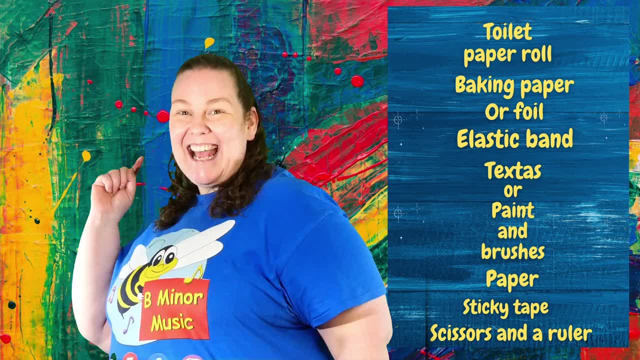 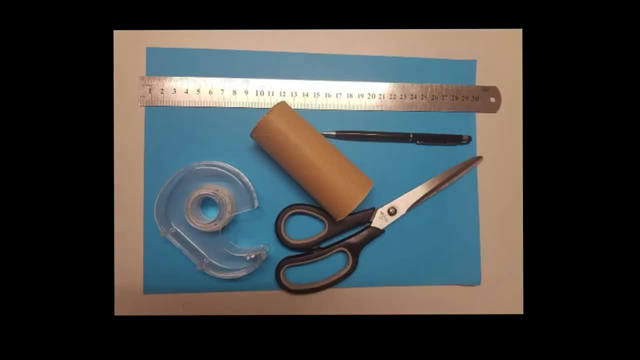 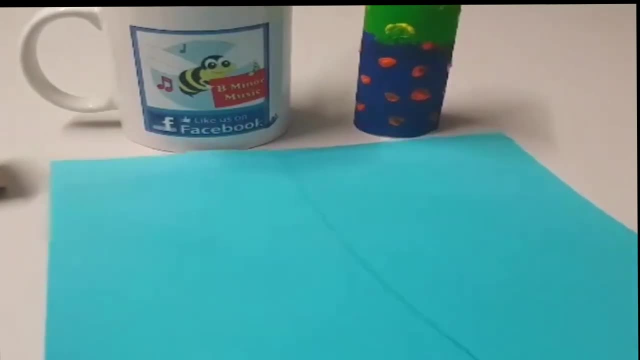 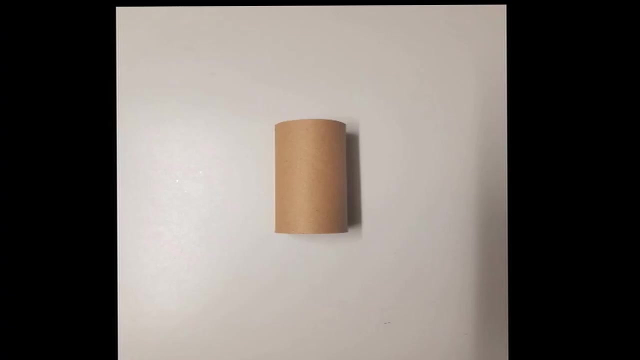 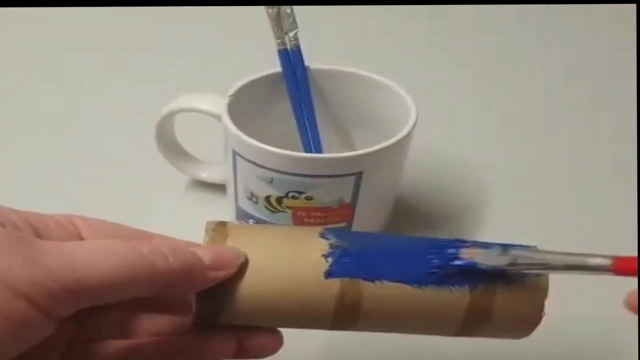 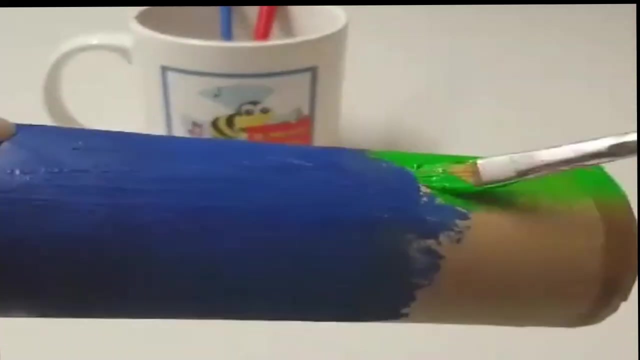 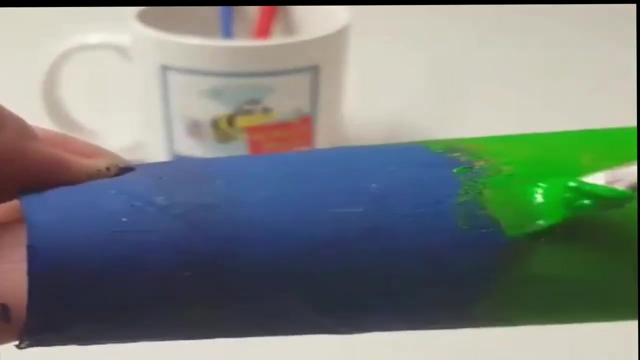 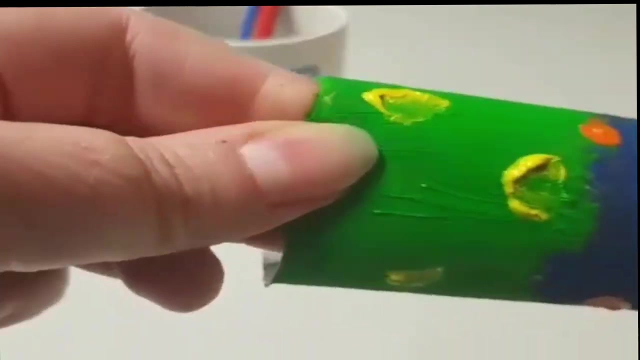 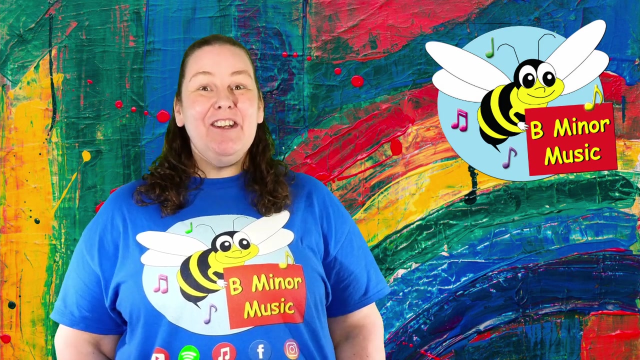 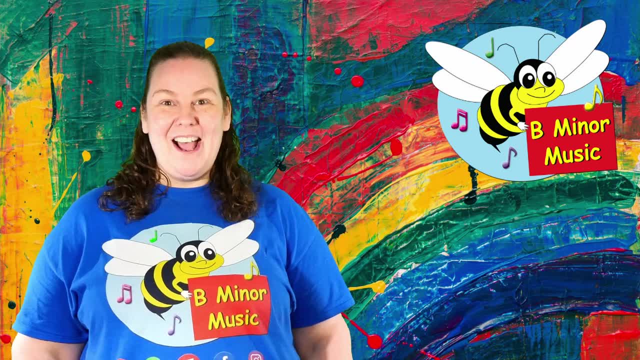 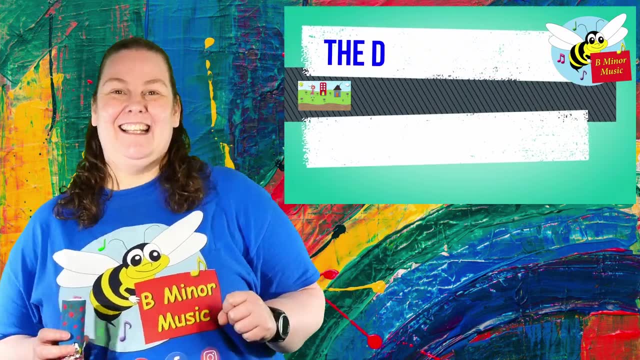 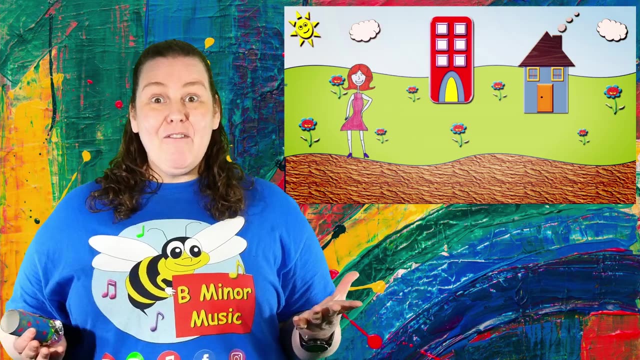 such a great job. all right, so we've got our kazoos and now it is time to play them. so are you ready to go? have you ever heard a song? it's a silly kind of song. it's a dibble, dabble, ding, dang bonkers song. 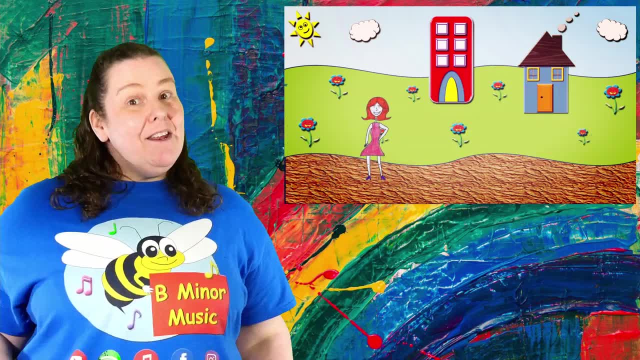 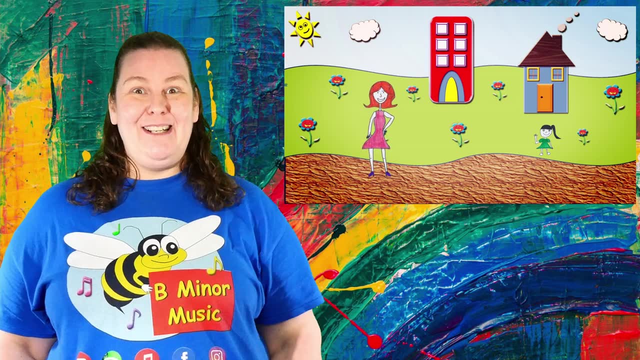 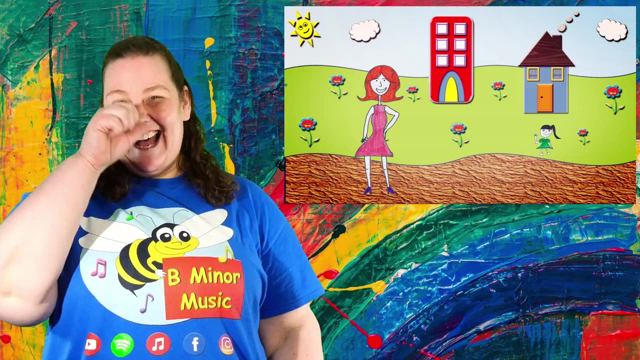 i was walking down the street and who was i to meet? it was a very special kind of girl. she was only very small and made me feel quite tall. then she began to speak. she croaked like a frog and snorted like a hawk. then she croaked cock-a-doodle-doo. 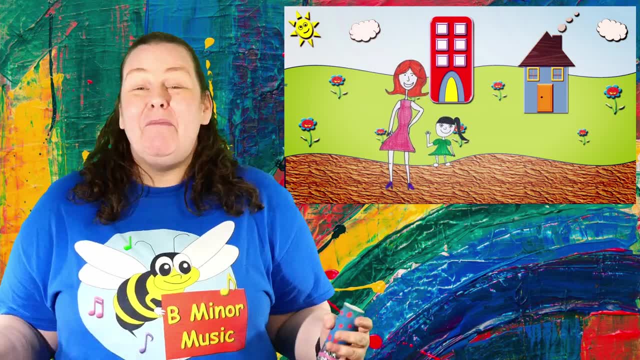 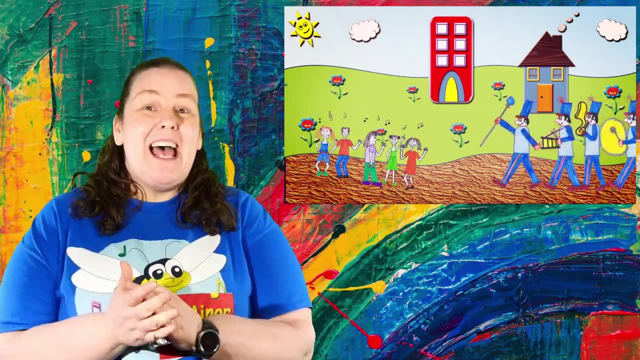 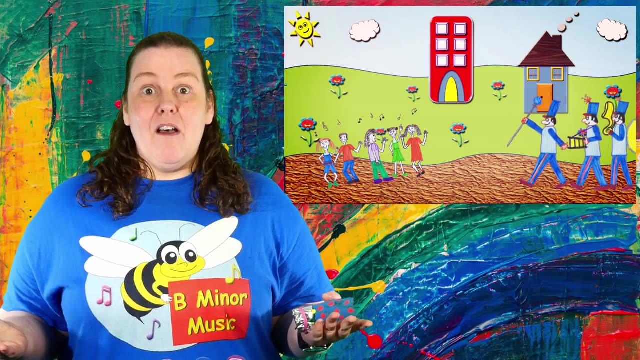 so i turned to her and smiled and then we both went wild as the band played dibble dabble doo. so it was the dibble dabble ding dang bonkers song, where the people laughed whilst they danced along. i have never, ever, heard such crazy, crazy words until the dibble dabble bonkers song. 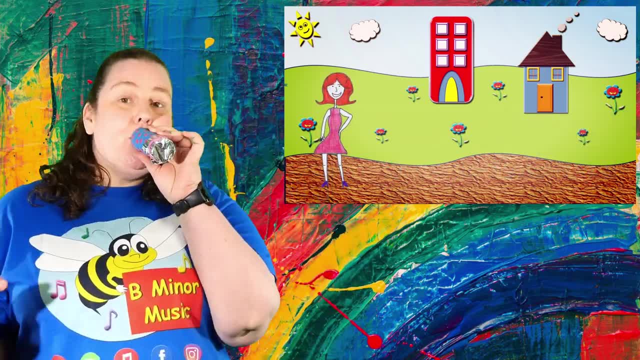 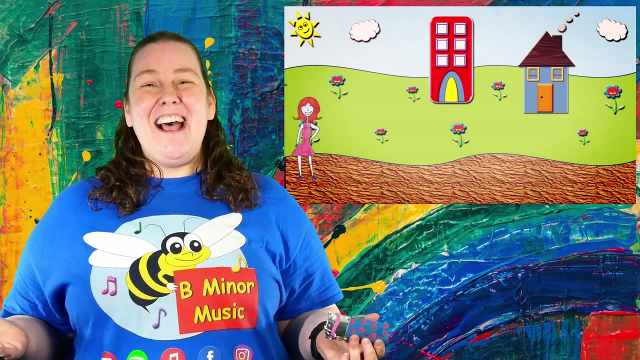 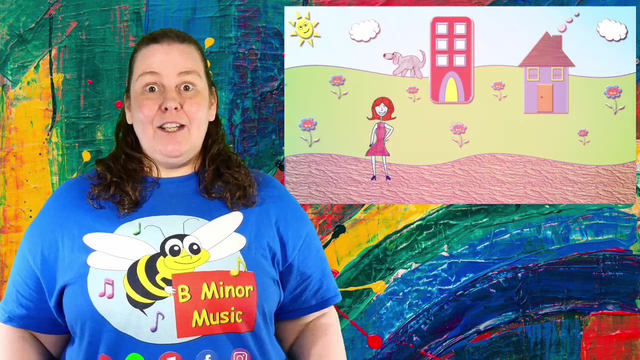 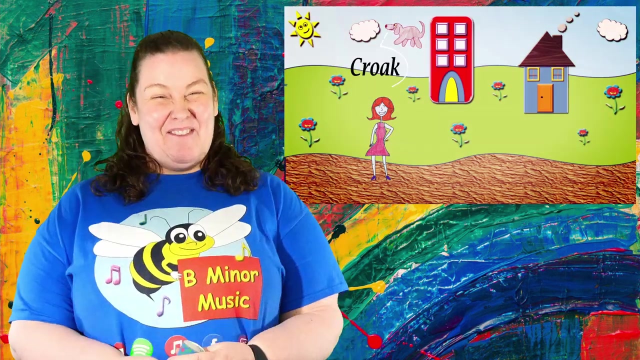 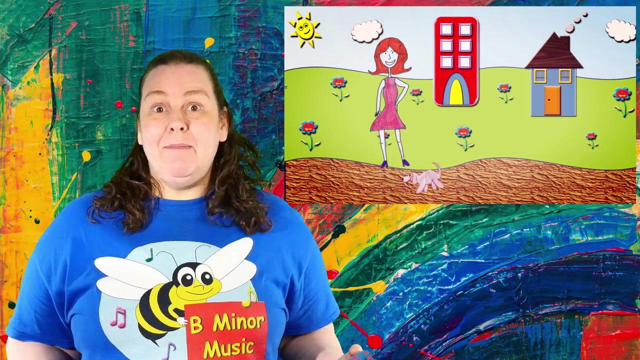 as i looked around the place i saw a man from outer space. he was doing the chicken dance. then it died and then the frog began to fly high up in the sky and i watched him float up in a trance. then he croaked like a frog, almost started like a hog. then he croaked cock-a-doodle-doo. 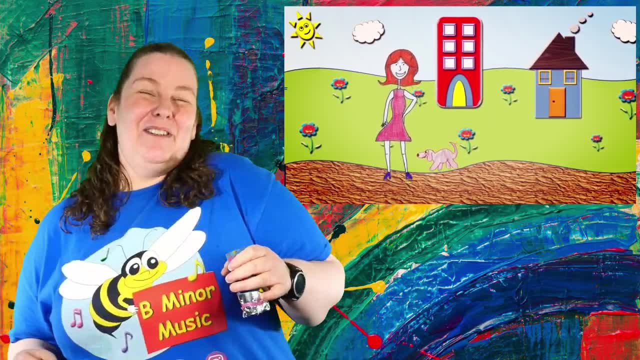 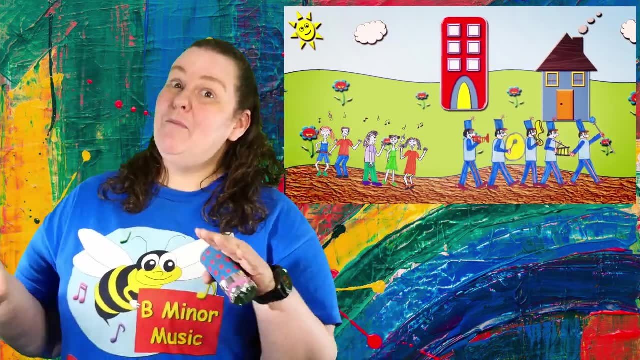 so i turned to him and smiled, and then we both went wild as the band played dibble dabble doo. it was the dibble dabble ding dang bonkers song where the people laughed whilst they danced along. i have never, ever, heard such crazy, crazy words, until the dibble dabble bunks came flying up on him. 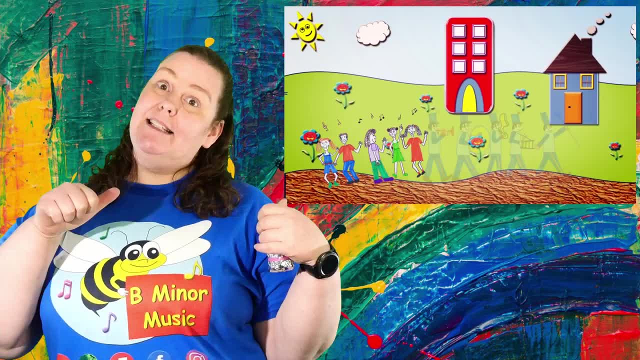 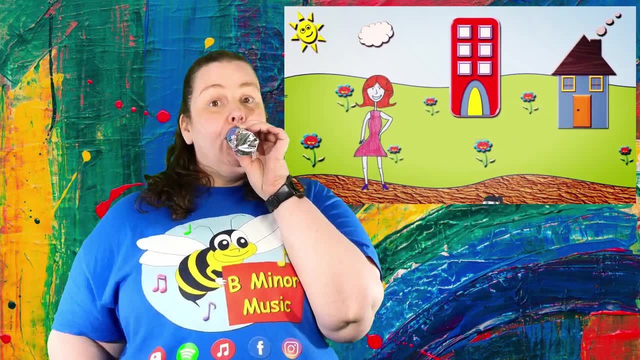 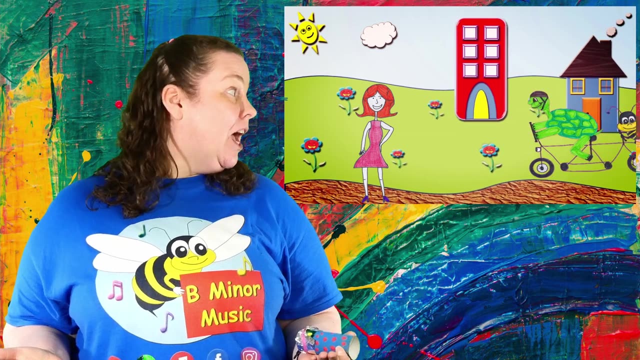 then he croaked like a hip-hop and he busted open the door of the tin environment where he was playing the music all over the place. Such crazy, crazy words, until the dibble-dabble-bonged his song. Now what was I to see? It was a turtle and a bee on a bicycle made for two. 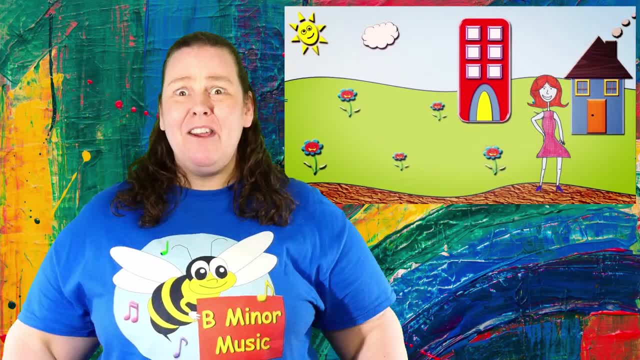 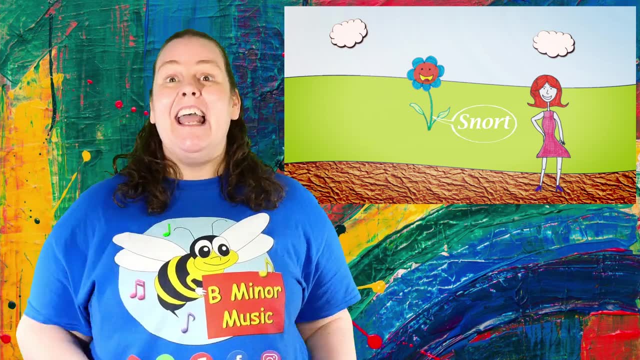 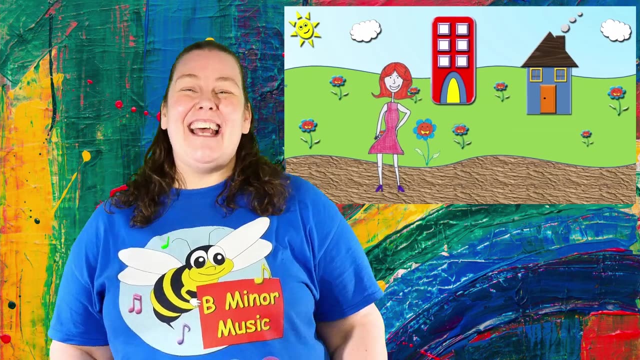 Then I looked upon the ground and was shocked at what I found. It was a cloud playing peek-a-boo. Then it croaked like a frog and snorted like a hawk. Then it crowed cock-a-doodle-doo. So I turned to hear the smile and then we both went wild as the band played dibble-dabble-doo. 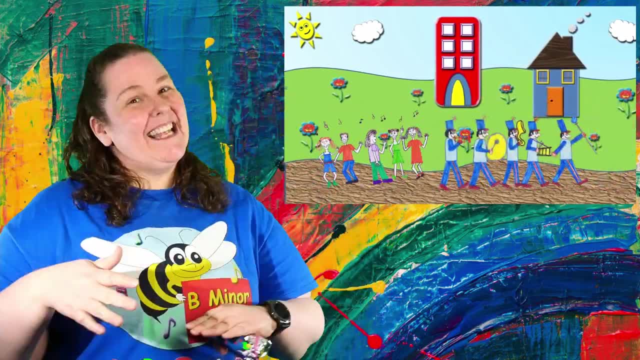 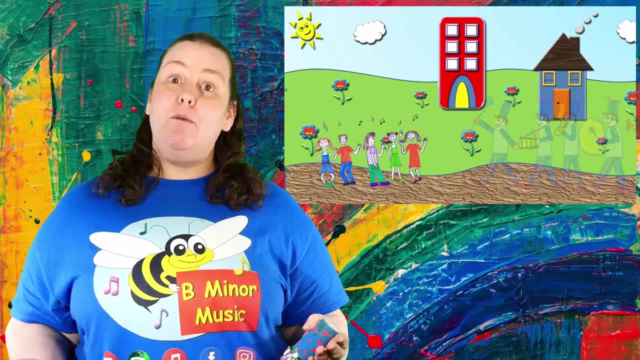 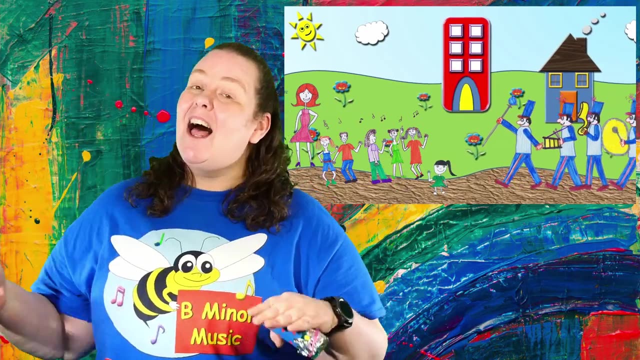 It was the dibble-dabble-ding-dang-bonged his song where the people laughed whilst they danced along. I had never, ever, heard such crazy, crazy words until the dibble-dabble-bonged his song. It was the dibble-dabble-ding-dang-bonged his song where the people laughed whilst they danced along. 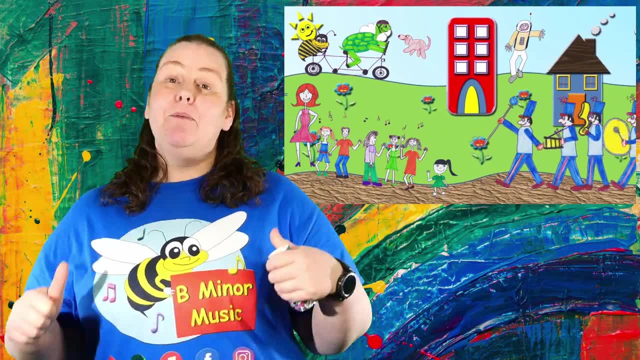 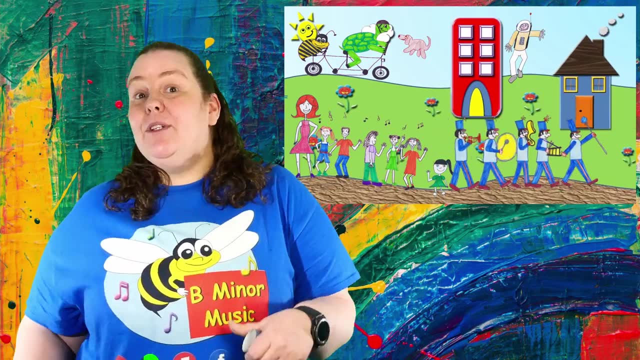 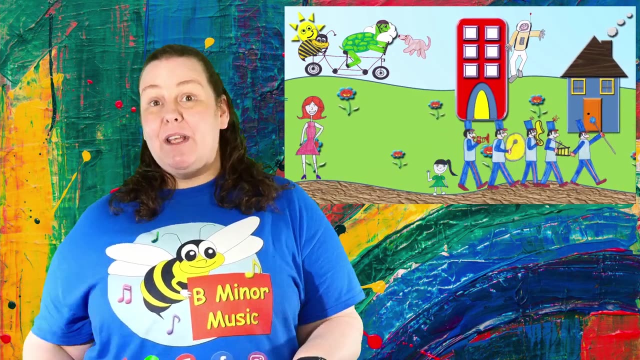 I had never, ever heard such crazy, crazy words until the dibble-dabble-bonged his song. I had never, ever heard such crazy, crazy words until the dibble-dabble-bonged his song. I had never, ever heard such crazy, crazy words until the dibble-dabble-bonged his song. 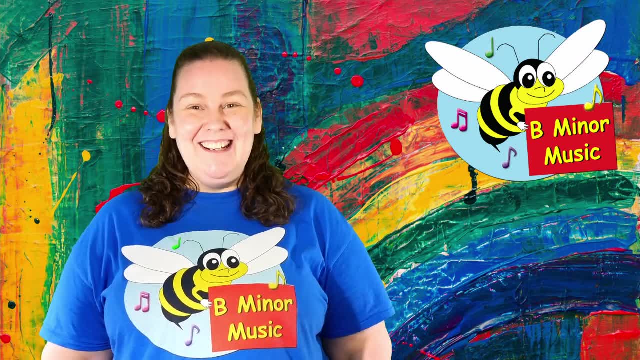 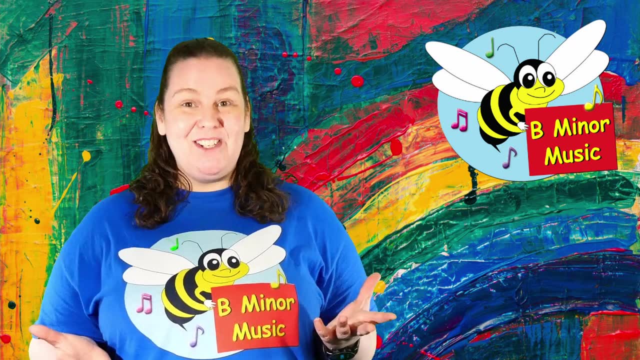 Wow, that was so much fun. Did you have fun too Now? if you enjoyed yourself, I'd love to hear all about it in the comments section. And also, if you took any videos or pictures of yourself making the kazoo or playing the kazoo, I'd love for you to hashtag B-Miner Music.